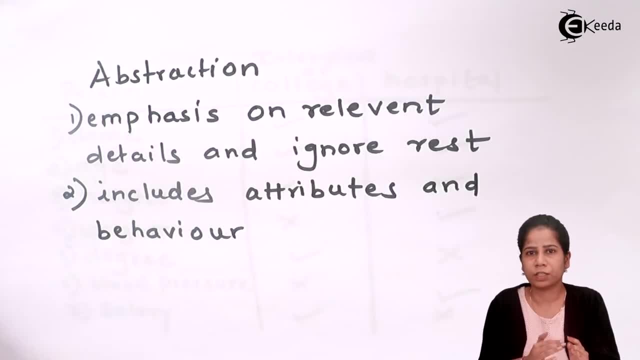 Okay, for example, if I am seeing a particular person, this person may be having some, he may having some educational qualification. It may he may having, or he or she may having, some height, some weight, some degree, Right, Some, what I can say, features. 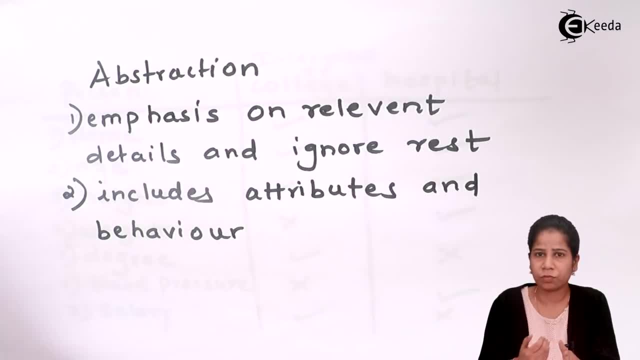 Okay, then it also perform some kind of behaviors. It shows some kind of behavior Like it can move in some way from one place to another, it can talk, it can read and so on. right, so all these features that one particular object is showing, all this feature does it? 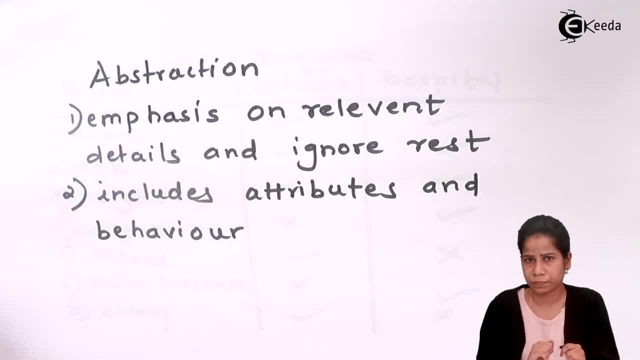 relevant at different situation. let's take an example. what do you mean by situation? what is mean? what do you mean by environment? now I'm considering this particular person. okay, this person into two different situations. okay, now let's take an example. this person is in right now, is in college. okay, this person, if I 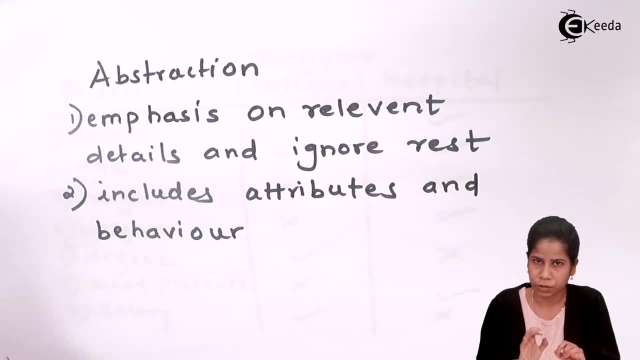 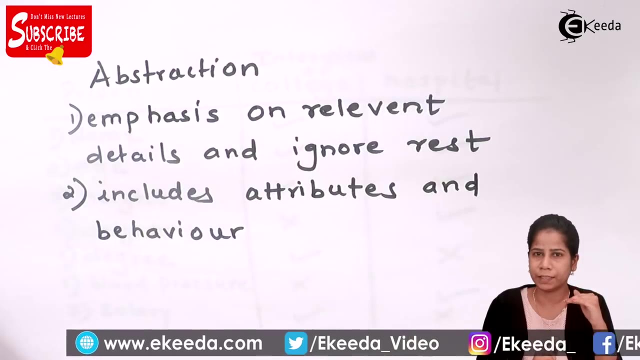 want this person to be admitted into the college. what are the things, out of all those listed attributes and behavior we require at that moment, for example, for taking admission into the college? first of all, I need the person's name. I need persons percentage. okay, then I may need, or what 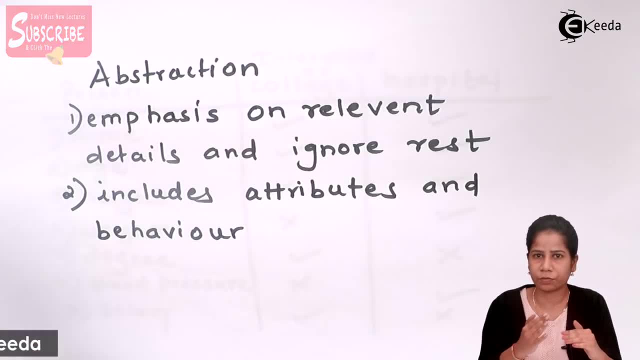 I can say it's marks on different subject or percentage. again, do it do that person's physical features- of height or a weight it required over there? no, it's not so. that is known as a situation, and in that situation there are only few features or behavior. 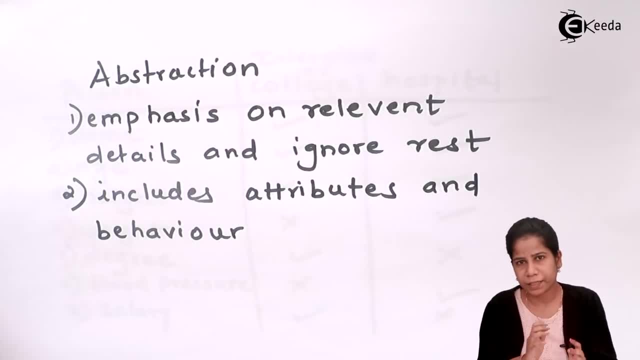 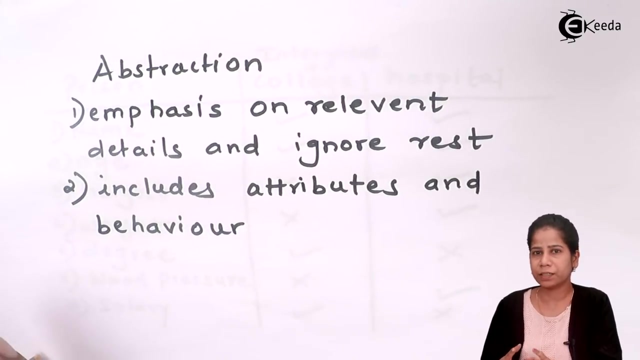 relevant at that point. okay, so that is nothing but an abstraction. abstraction talks about only concentrate on the relevant thing and rest of the thing should be ignored. okay, so abstraction is nothing but an abstraction is nothing but emphasizing on relevant details and ignore the rest, and abstraction it. it is possible in terms of attributes as well as in terms. 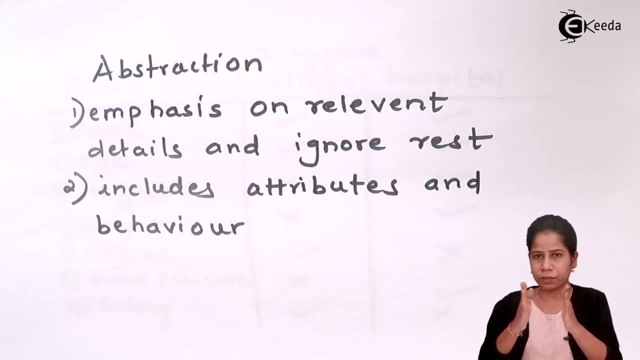 of behavior, what I mean at attack at a given environment. I am going to emphasize on certain attributes as well as some behavior as well. in a college, or what are the required behaviors for the person is required first of all, it's reading capability, right, or learning capability is more important. all other 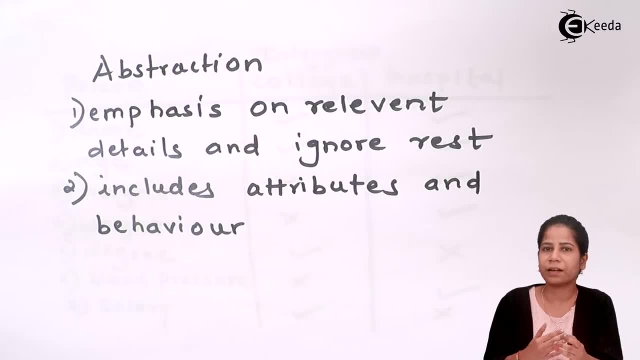 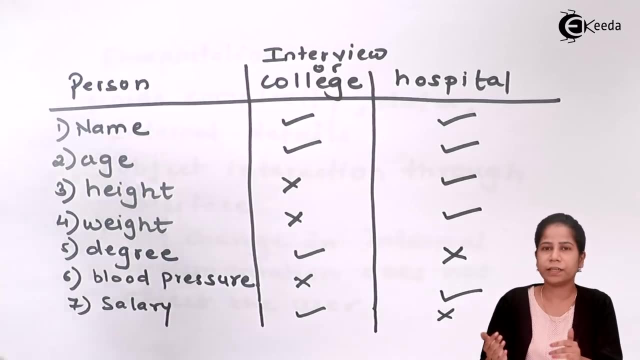 abilities that particular person is having are irrelevant at that particular situation. okay, so that is nothing but an abstraction. let's see example of abstraction. so here I am having a person. this person is having certain attributes. okay, so for the attributes like name, age, height, weight, degree, blood pressure. 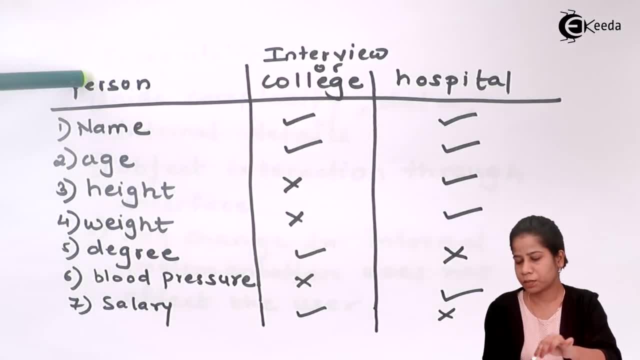 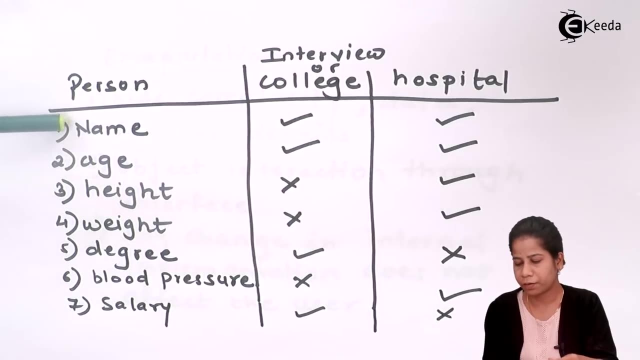 salary. and the third one is the person's ability to do the job, and I am going to, etc. now I am considering this person intake in admitting into the college and admitting him into the hospital. now, the in first situation, what are the relevant things? I am Rick. I required, though so name. yes, it is required for a college. 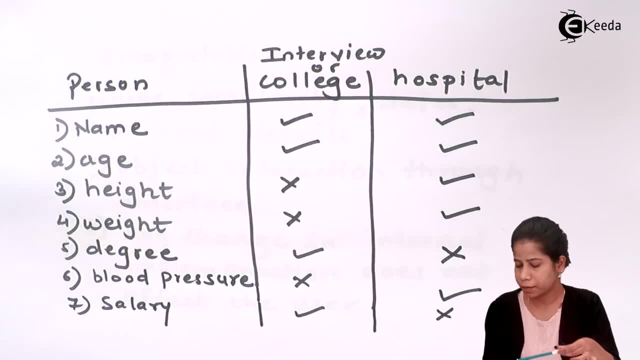 age is required. height and weight doesn't matter over there. degree, yes, it is required. what blood pressure or blood group it have, it doesn't require over there. so as the salary now we will consider this person into admitting into the hospital. so in that case, definitely I will be requiring his name, his age, his 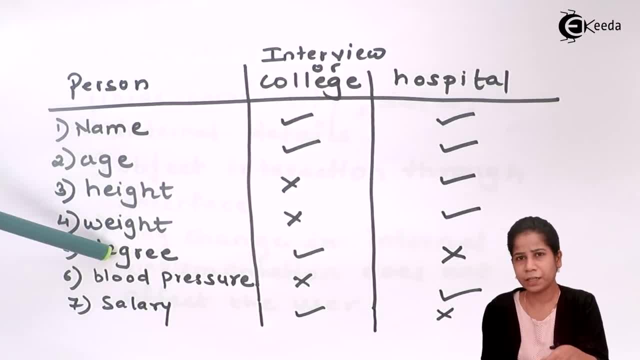 height, definitely his weight degree. don't require blood pressure or blood group. yes, it is required, or salary may not be required. okay, so this is nothing. but in a different situation, what are the relevant things? and there, and we are emphasizing on those relevant things, okay, that is nothing. 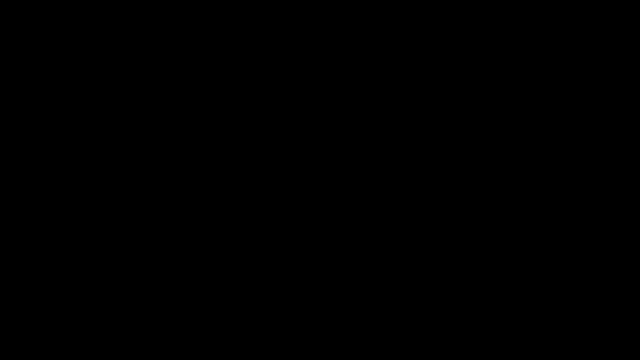 but an abstraction. thank you,